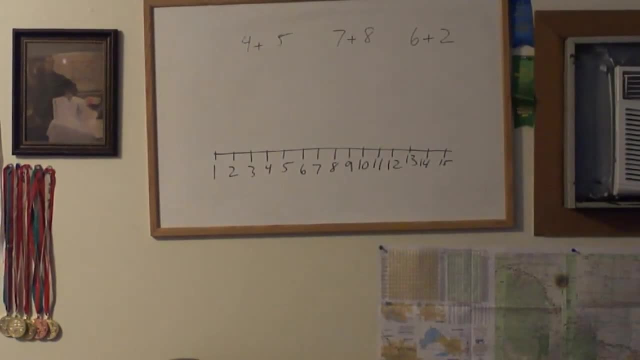 Hi everyone, and welcome to another lesson to Eureka Tips for the computer. 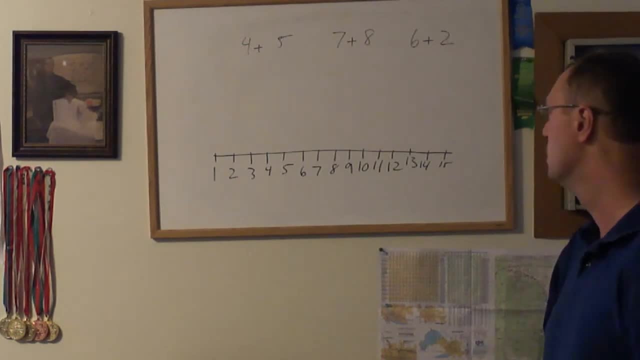 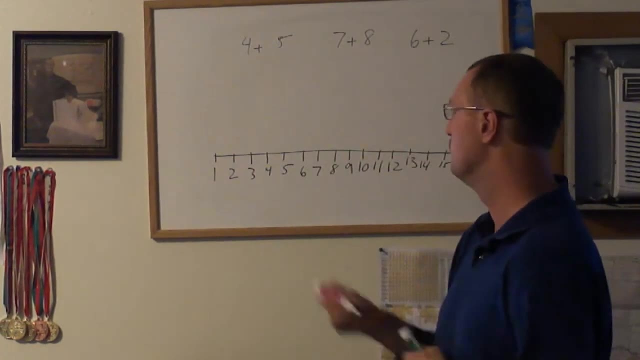 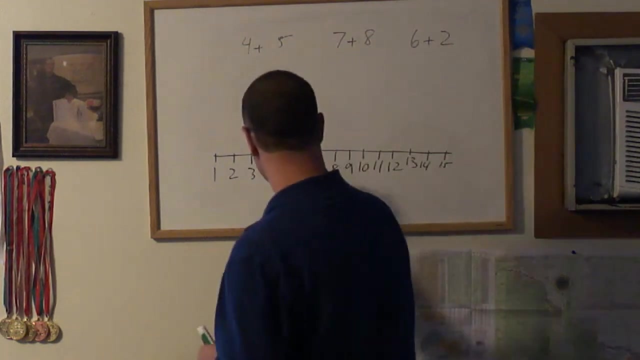 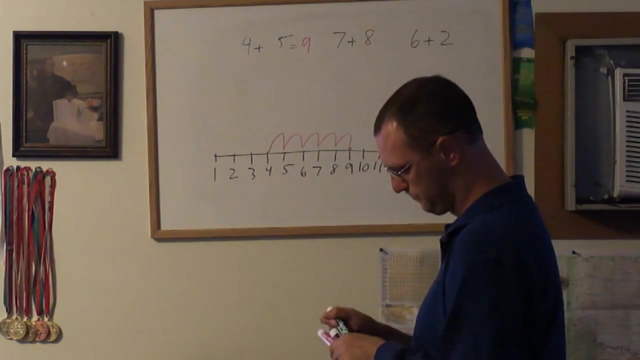 I'm actually trying to use the number line to find the stone for each. So to start, I'm going to use the paint to find the stone. Use the number line for four plus five. We're going to start with four. We're going to increase five. One, two, three, four, five. That's equal to nine. Now, let's do three for the next one. 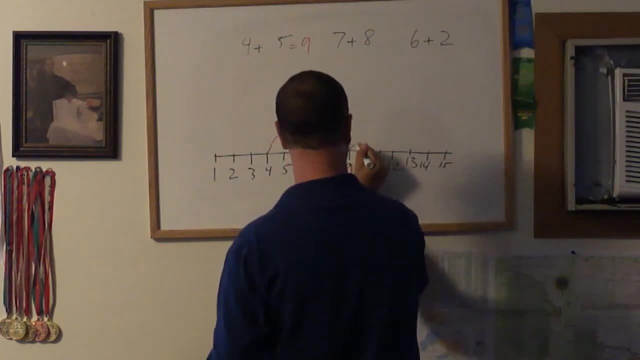 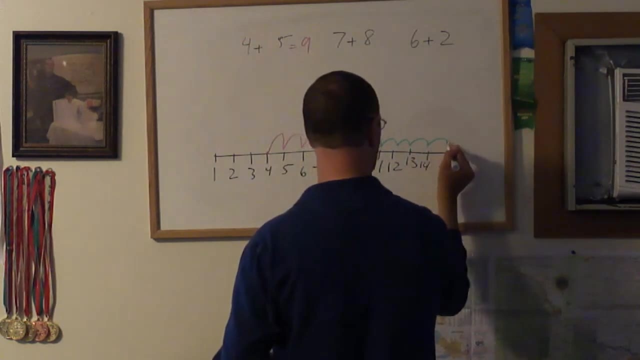 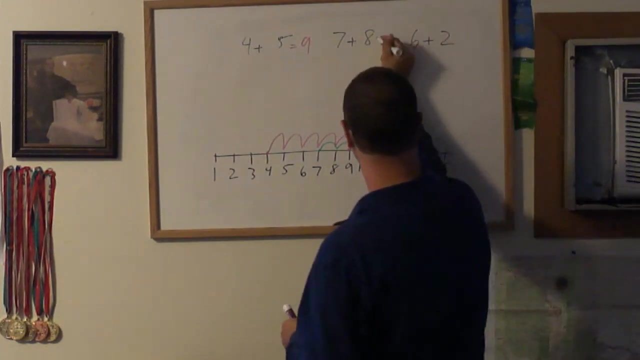 So that's one. Two, three, four, five, six, seven, eight. Seven plus eight equals fifteen. And I know it's all equal, so I'm going to use the number line anyway. 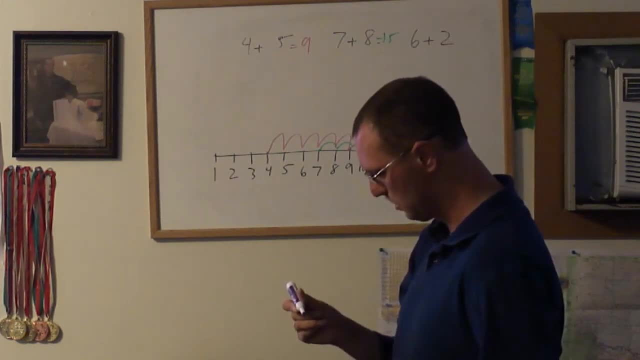 And we'll use the violet color as well. 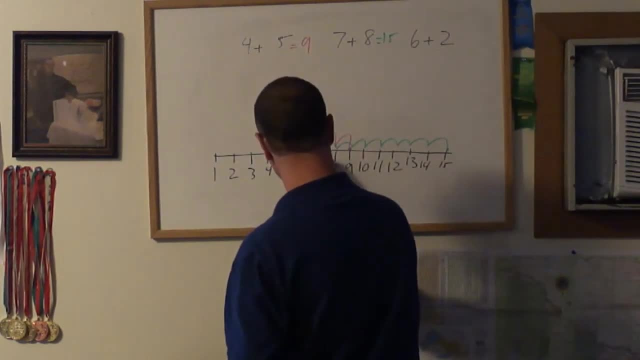 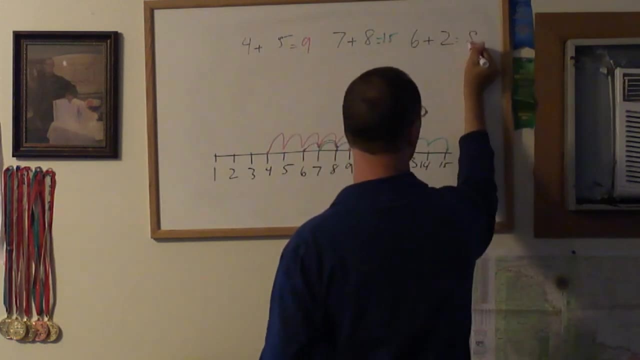 Six plus two. So it's six. One, two. Equals eight. 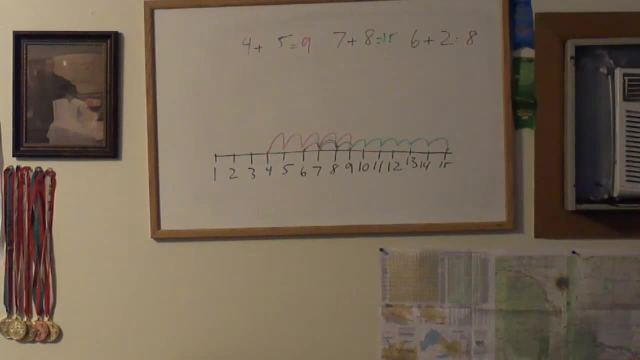 All right. That's the answer for the short play here. We're going to start for the next one. 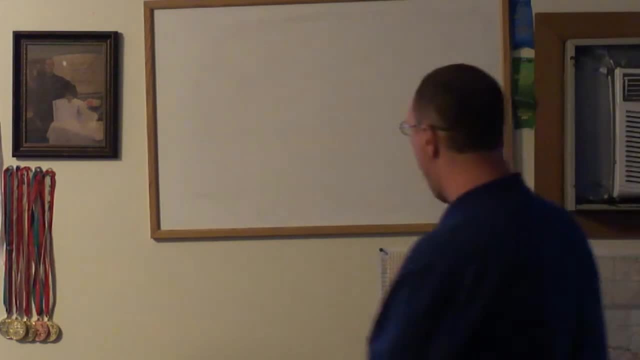 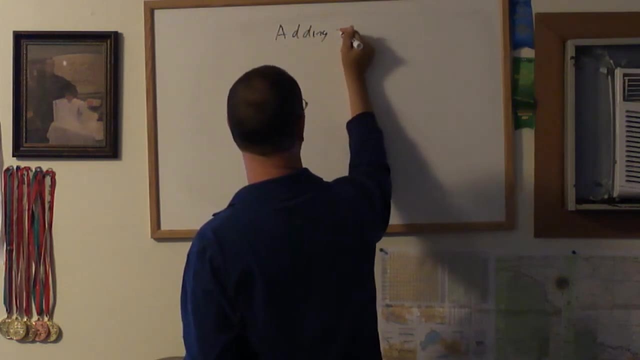 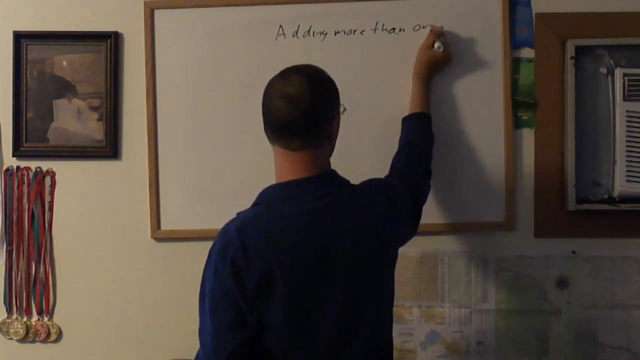 All right. I hope I have more than one digit. 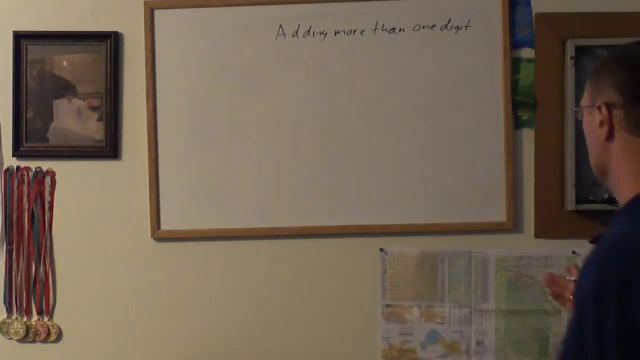 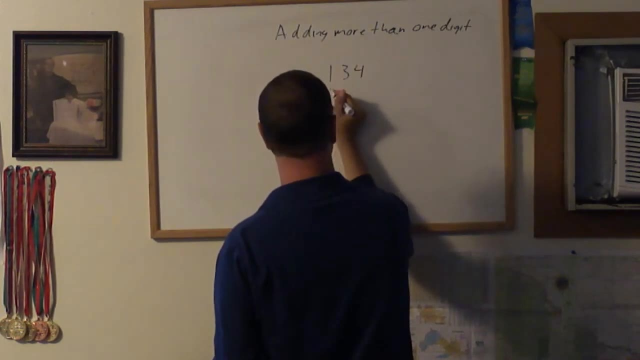 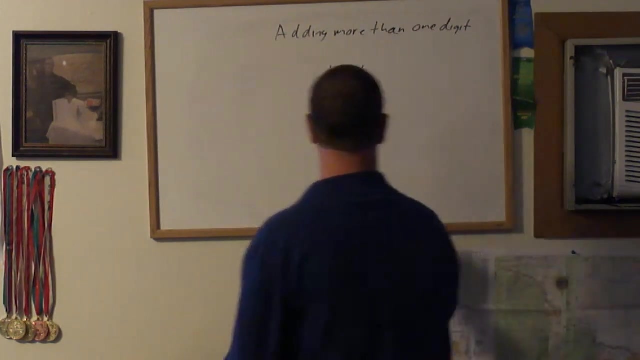 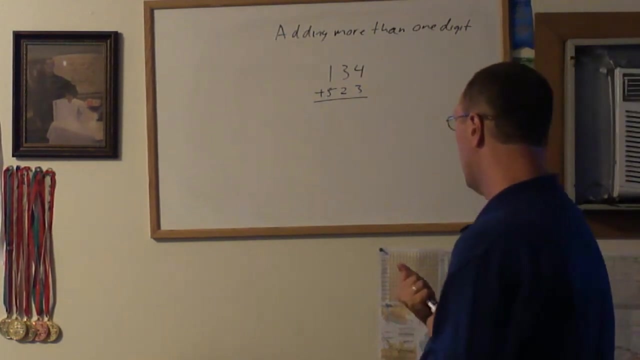 Let's kind of start off with a problem here. We'll start with 134. 134 plus 523. This is how I do it. 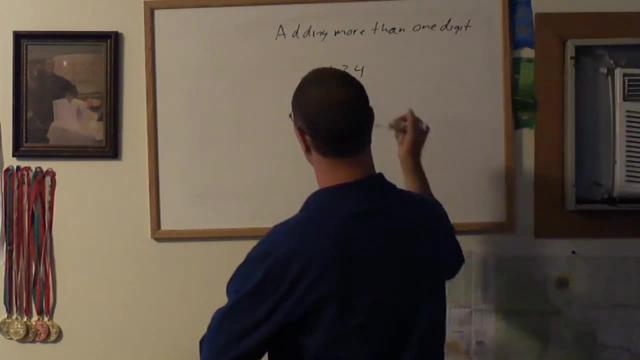 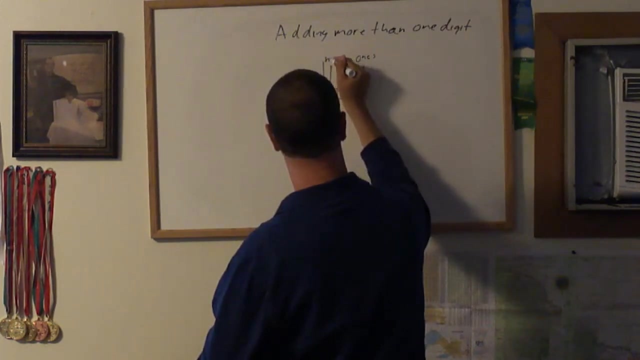 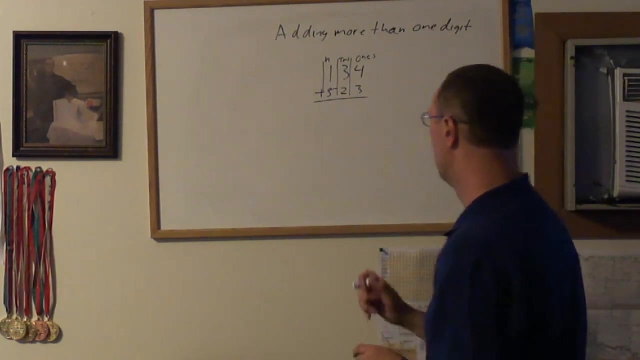 I go to the one place right there. The one. Ten. Hundred. I start with the one place. 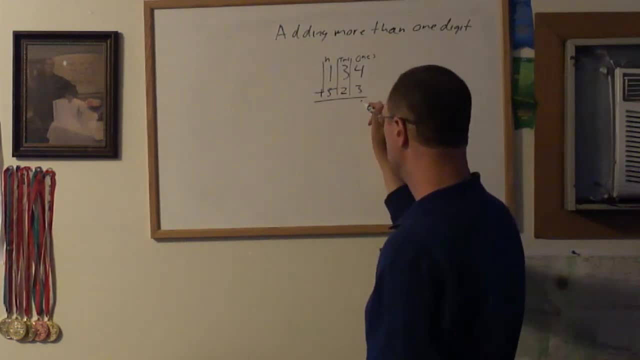 Four plus three is equal to seven. 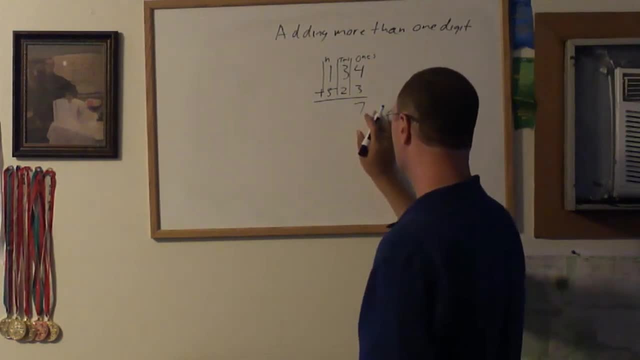 Seven richter. Seven richter and the one place. And I go to the ten. 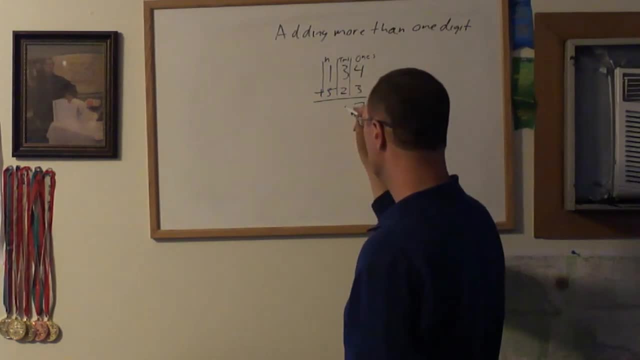 Three plus two is equal to what? Five. 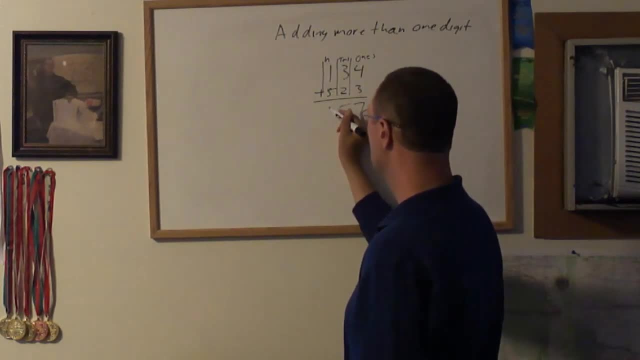 And then to the hundred. One plus five is equal to six. 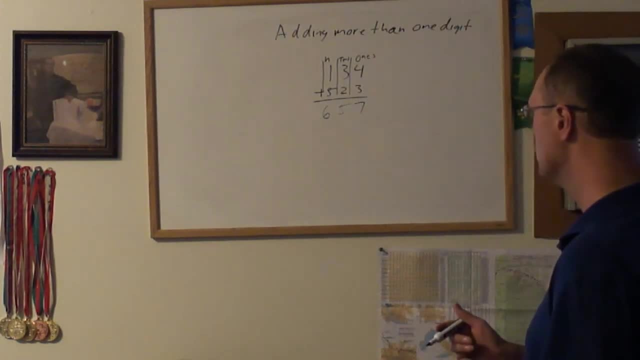 And now I have an answer. 657. 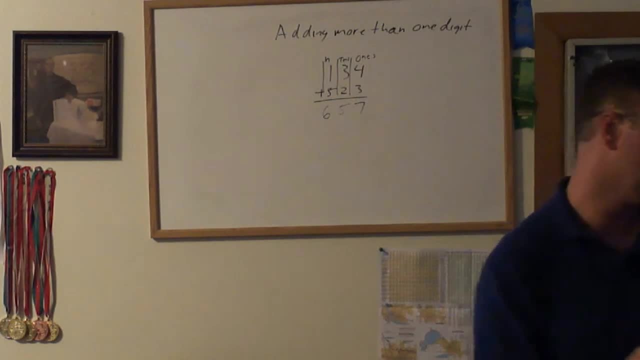 Now that is just a simple addition problem. Now let's try something a little more harder. Let's try it. 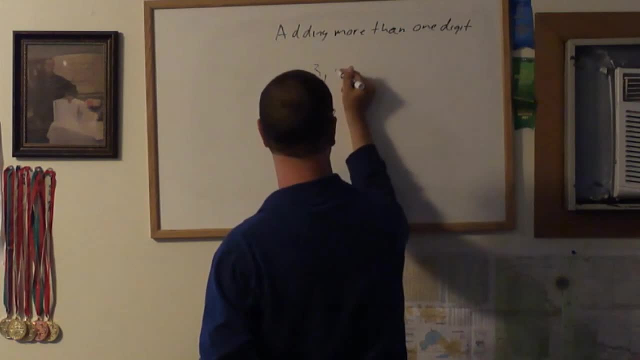 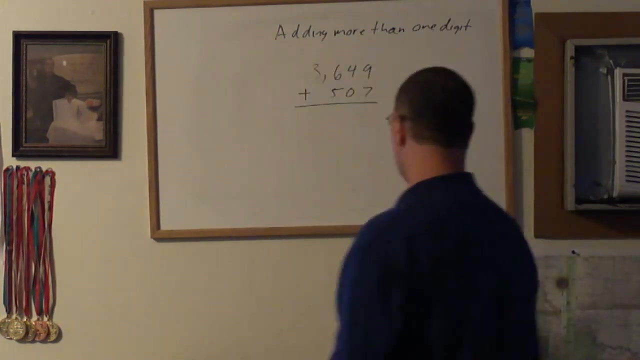 Let's try 3649 plus 507. All right. 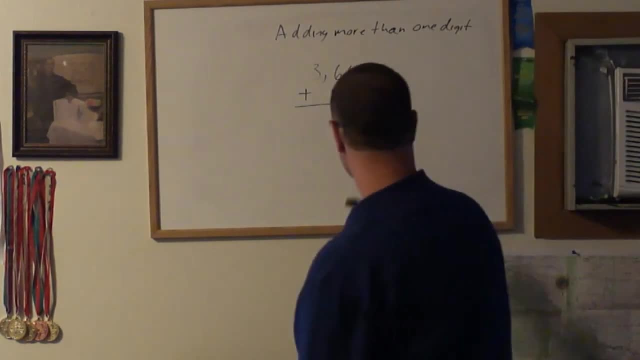 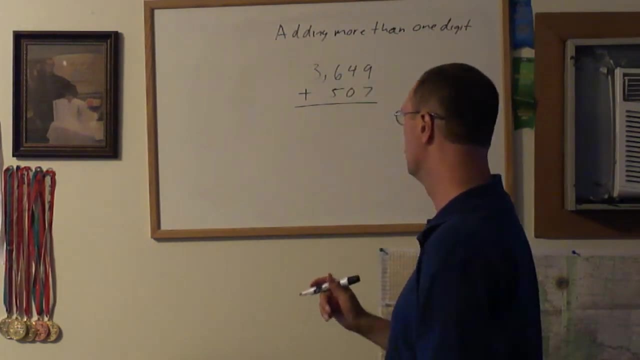 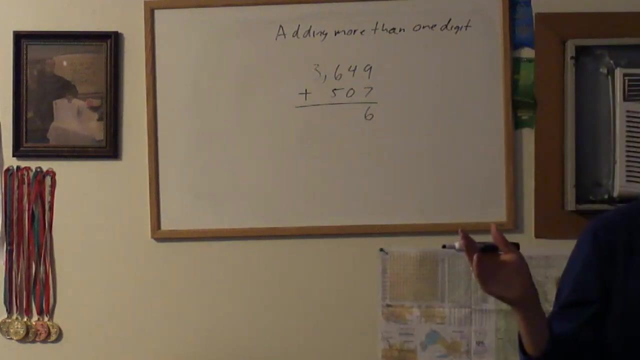 Same thing. We go to the ten place. Nine plus. Seven. Is equal to. 16. What is this? Now, you want to know where does the one go? Does the one go here? Um. 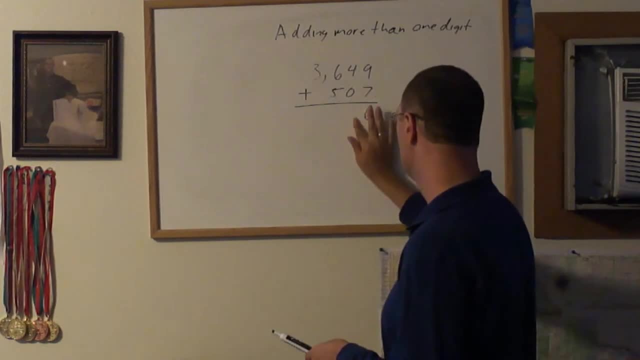 That's not in your mind, but it does not. 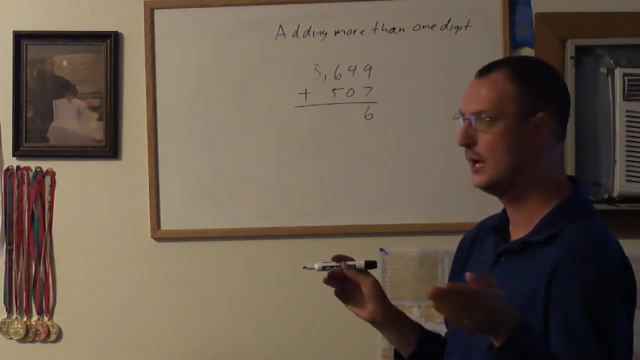 One is like a ten place. It's in the ten place. 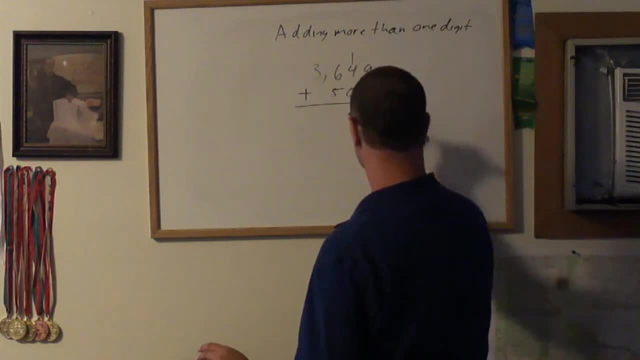 So I'll just put the one right there. I'll just put the one right there. 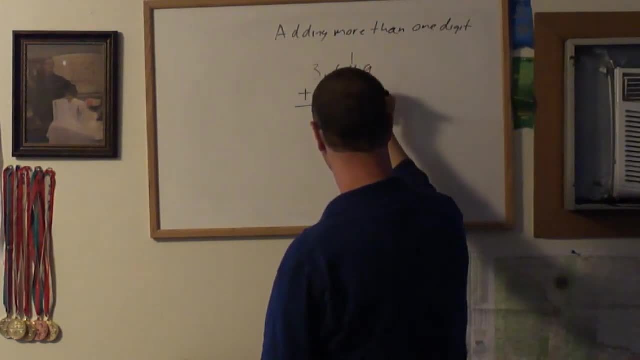 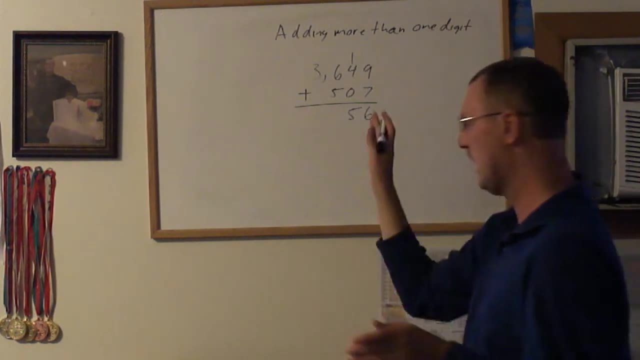 And I'll add the one to four plus the zero equals five. Now, that's just a six one digit. 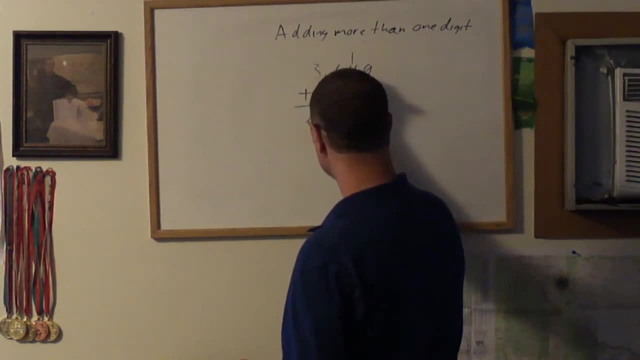 Now let's go to the hundred. Six plus five is equal to eleven. 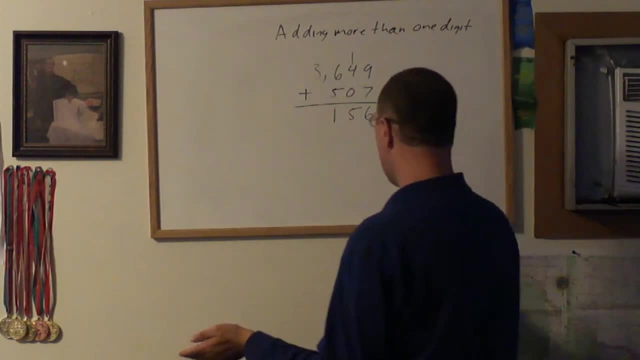 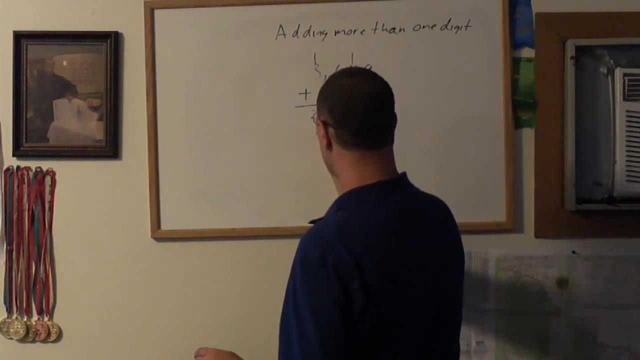 Again, where does the one go? In the thousand area. One plus three right there is equal to four. So we have an answer. 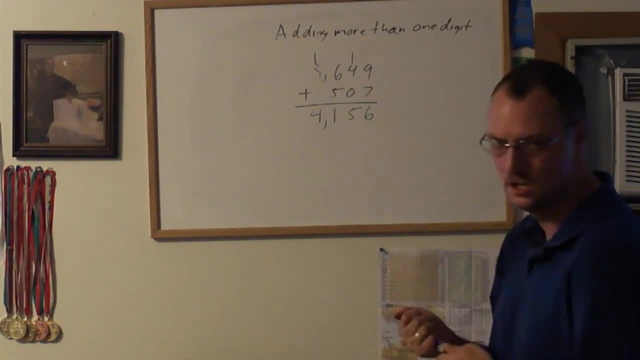 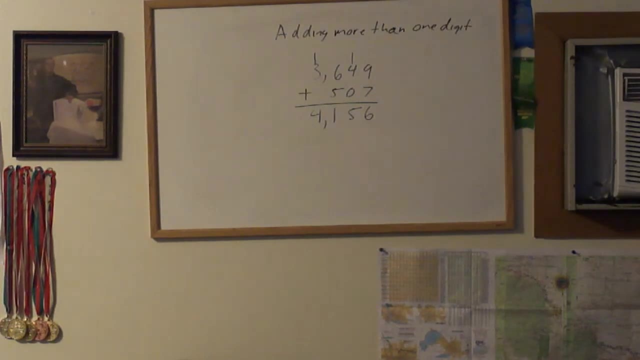 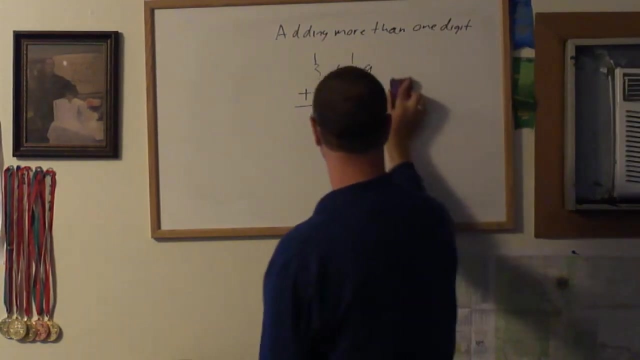 4,156. All right. That is the answer to the addition problem. 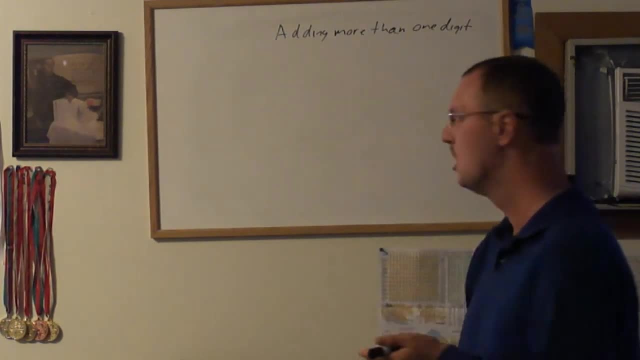 Now, we're kind of acting up. Just a little more to add another number. 1,037. 581. 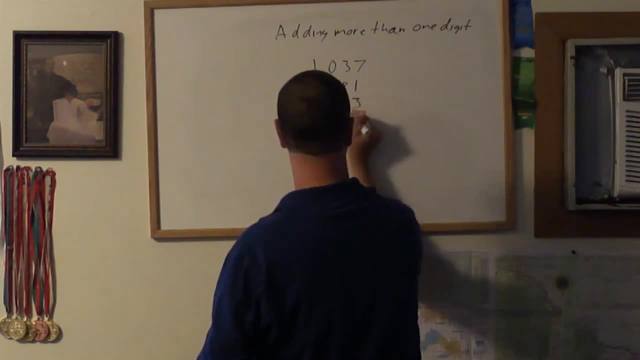 293. Let's add them up. Let's add these three numbers up. Now, we're going to add more numbers. It's going to get a lot tougher. 7 plus 1 plus 3. 3 plus 1 equals 4. 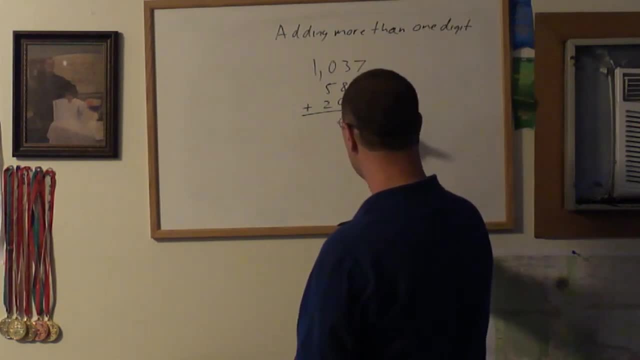 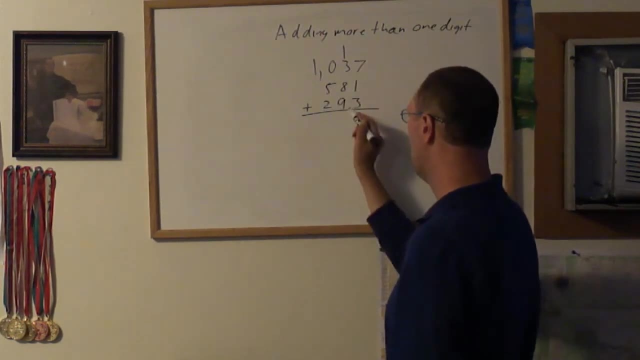 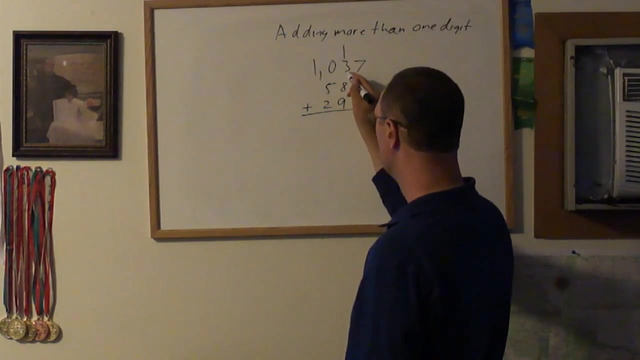 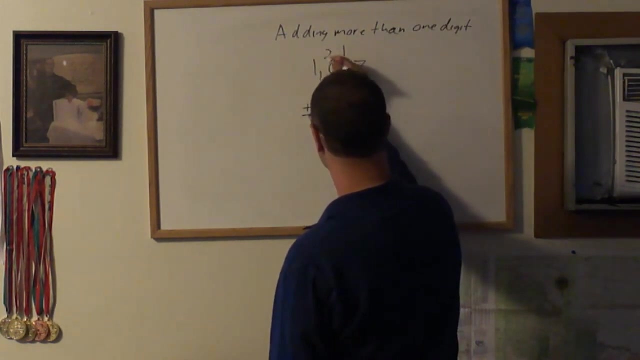 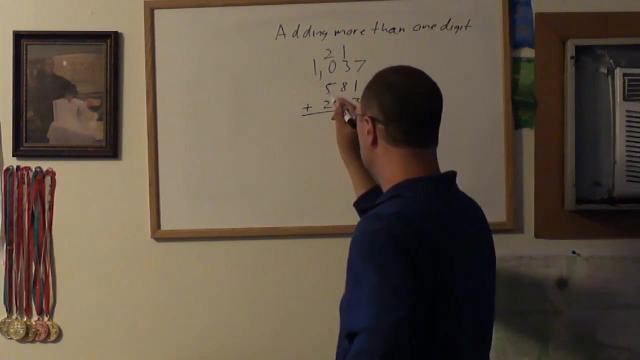 Plus 7 is equal to 11. And the one right there is in the digit. 9 plus 8 is 17. Plus 3 is 20. Plus 1 is 21. It carries 2 to the hundredth place. 5 plus 2 is equal to 7. Plus 2 equals 9. Nothing better. 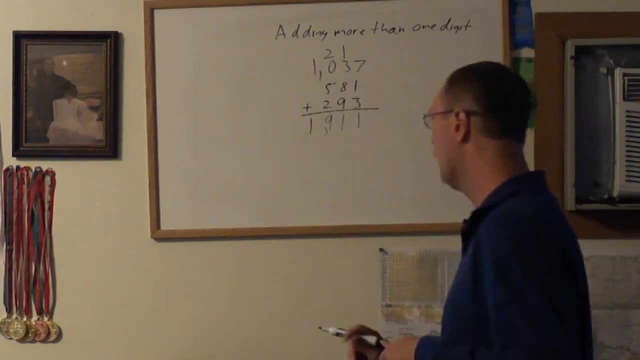 Let's add one more number. And we got 1,911. All right. 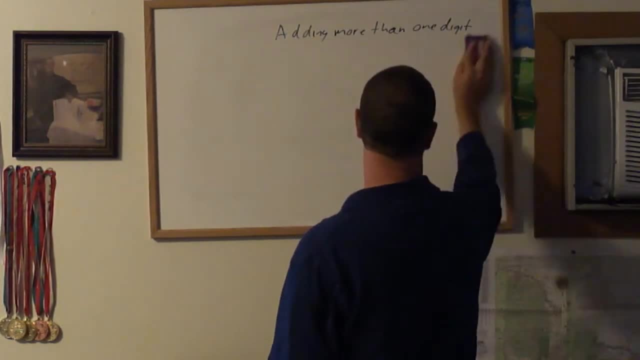 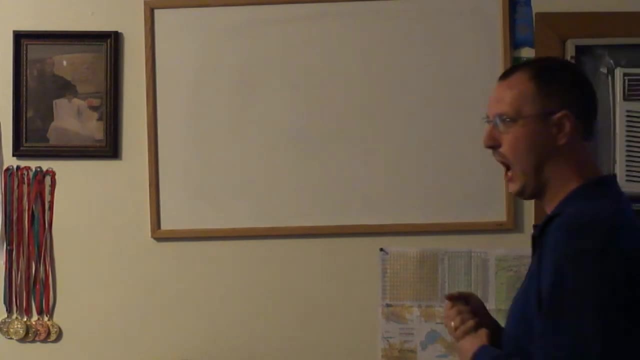 Now, we're going to have something a lot harder now. All right. All right. We're going to add one more number. Let's add it. 349,788. 13,409. 45,205. 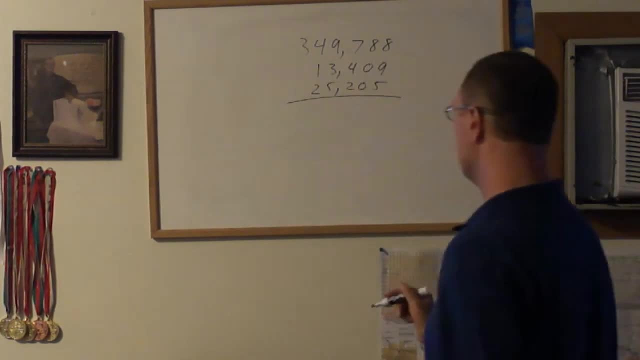 All right, let's add them up. 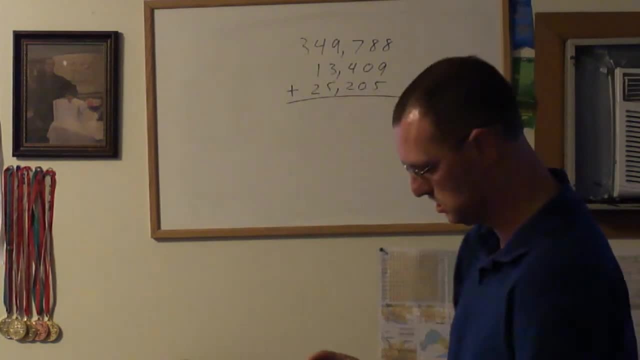 We need one more example before we switch. 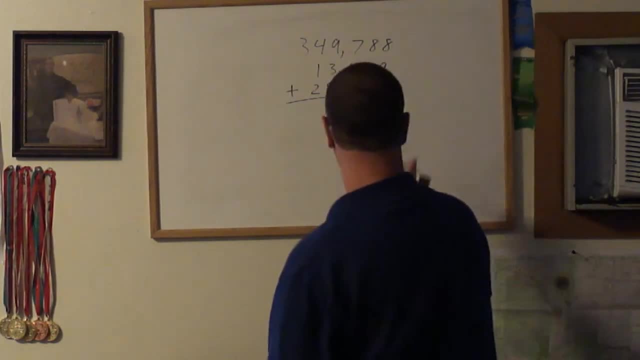 9 plus 8 is 17. Plus 5 is 22. 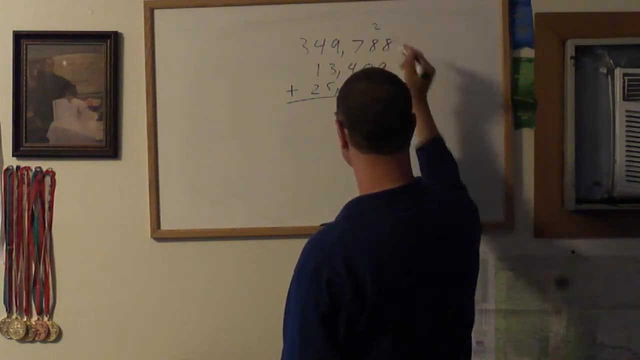 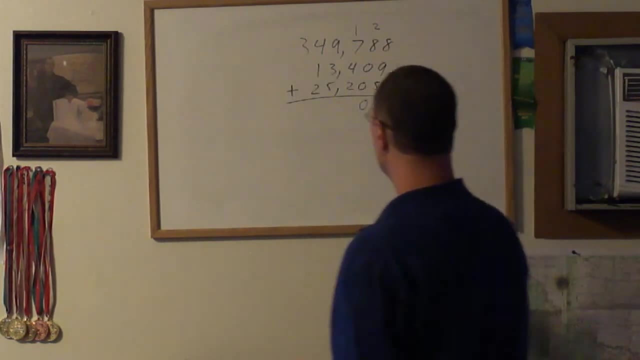 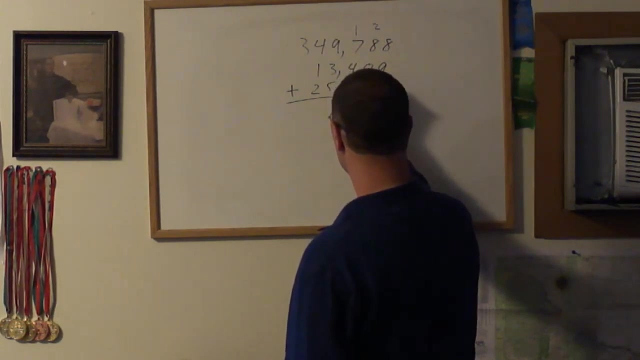 8 plus 0 plus 0 plus 2 is equal to 10. 7 plus 4 is equal to 11. Plus 2 is equal to 13. 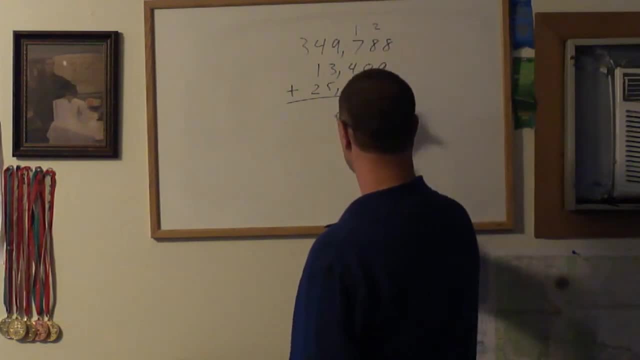 Plus 1 is equal to 14. All right, we're getting going here. 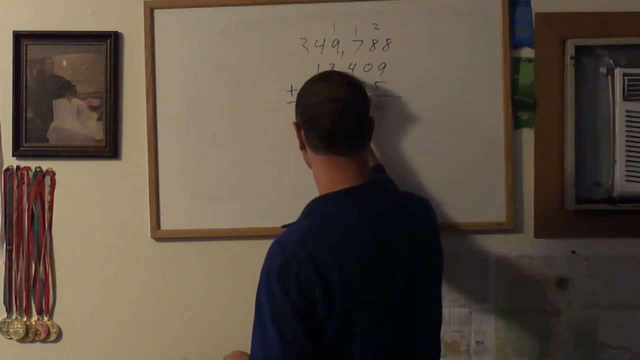 3 plus 5 is equal to 8. Plus 9 is equal to 17. Plus 1 is equal to 8. Plus 1 is equal to 18. What's the counter there? 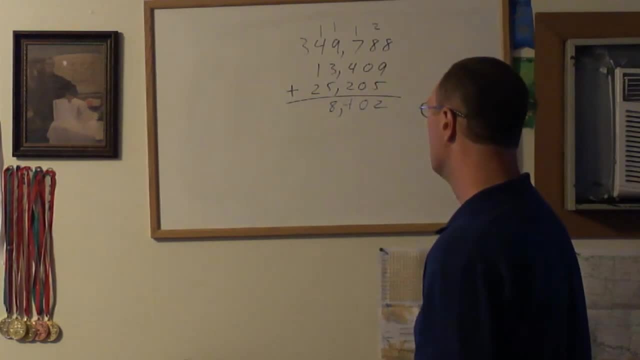 4 plus 1 is equal to 5. Plus 2 is equal to 7. 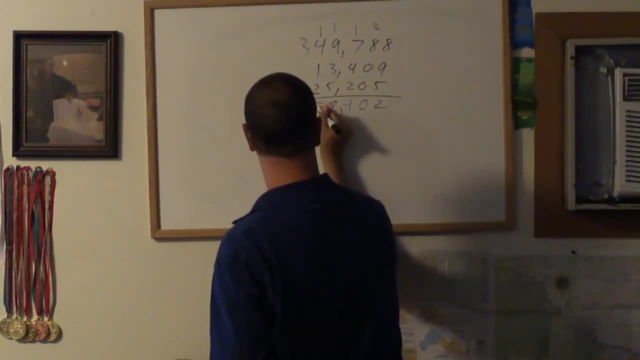 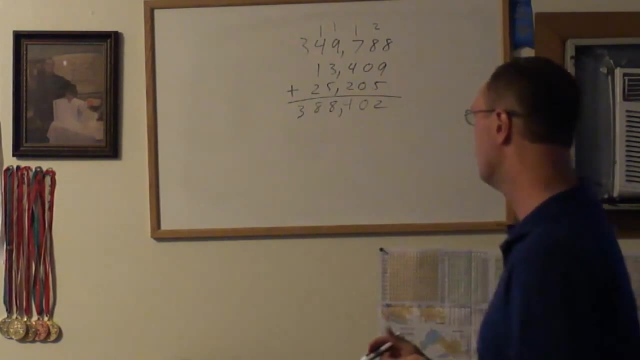 Plus 1 is equal to 8. And the 3 is right there. 388,402. 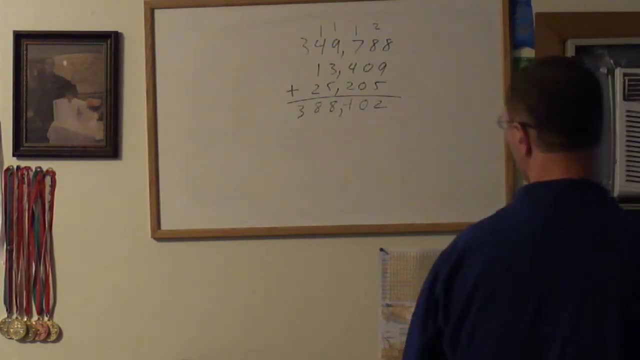 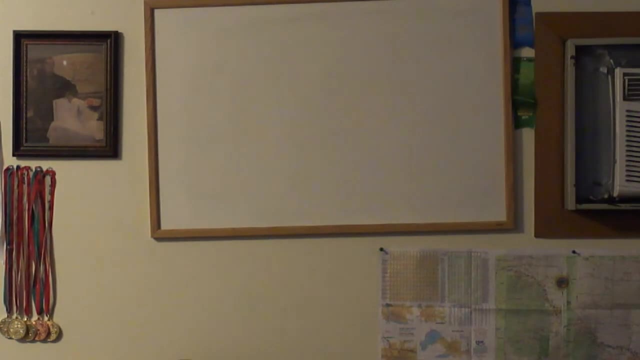 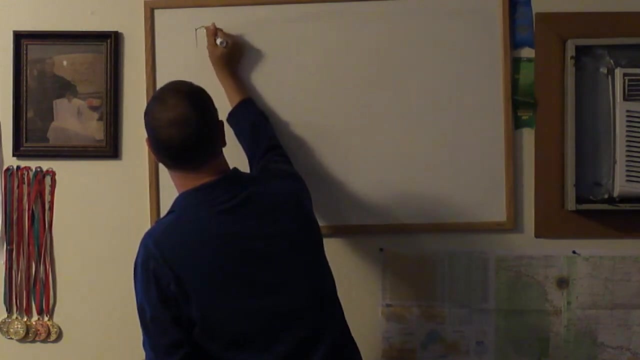 All right. All right, there's going to be four questions. There's going to be four questions this time. Find the sum. 1. 300. 22. 453. 2. 23,495. 57,087. 3. 2,495. 2,041. 2,238. 2,341. 2,341. 1,390. 2,391. 5,513. 5,513. And 4. 4,341. 4,141. And 4. 4,141. 4,341. 4,142. 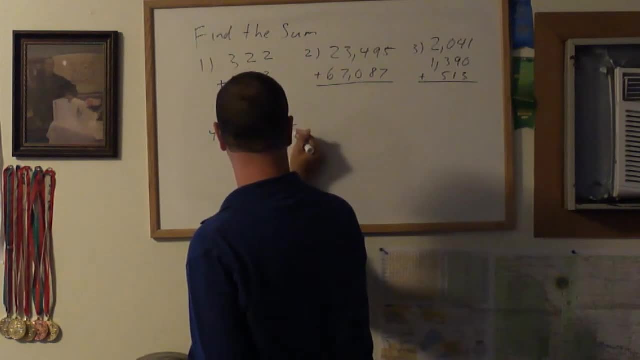 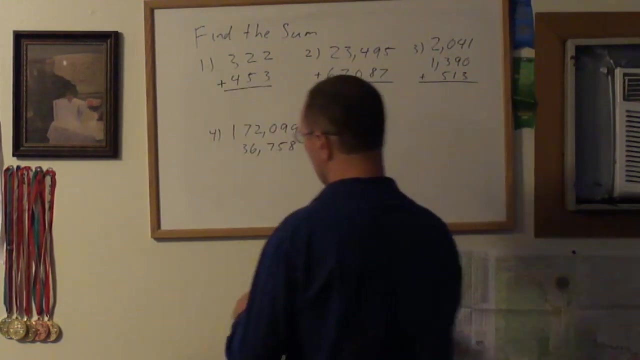 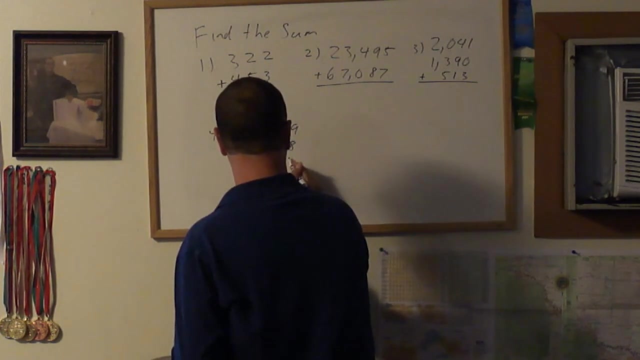 Thirty-two thousand, ninety-nine, thirty-six thousand, seven hundred and fifty-eight, eighty-one thousand, one hundred and seven. There you go. 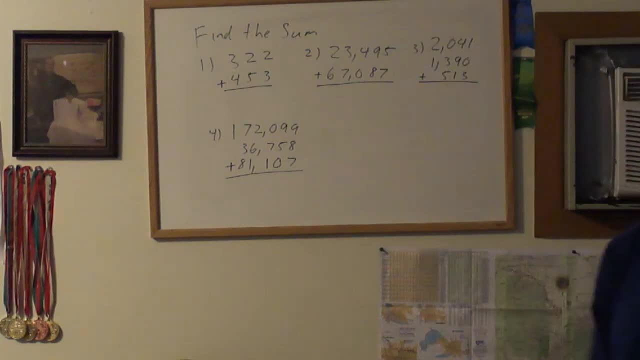 And that is the footage right there. If anyone can do it, it's fine. That would be just awesome. 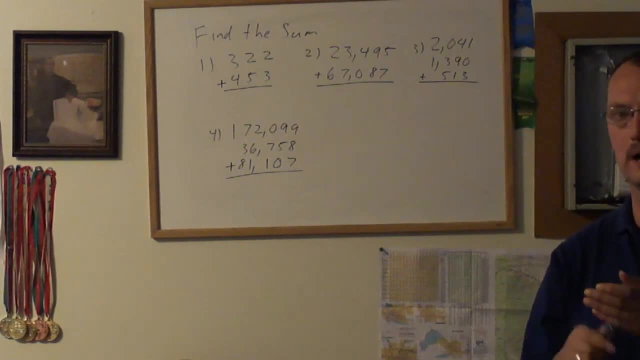 And tomorrow, we'll have a chance to do an introduction to subtraction. And coming up, I'm going to tell you the subtraction whole number. One more time, there's a quiz right there.